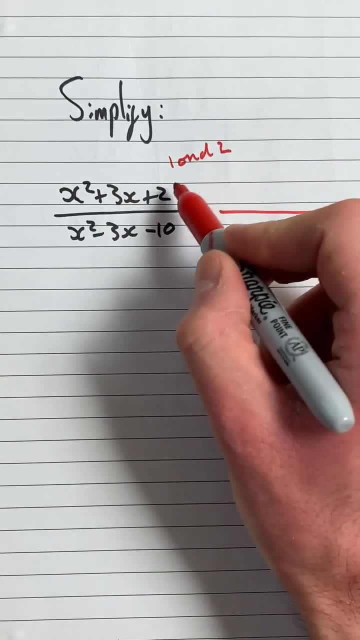 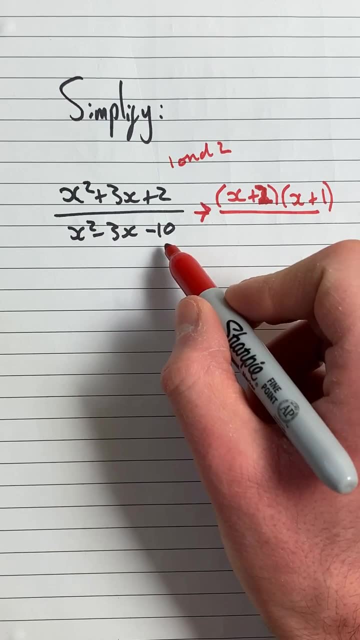 one and two. So we can factorise the numerator like this: x plus two multiplied by x plus one. Now let's repeat the same process in the denominator. We're looking for two numbers that add to make minus three and multiply to give minus ten. This one's a bit trickier, but 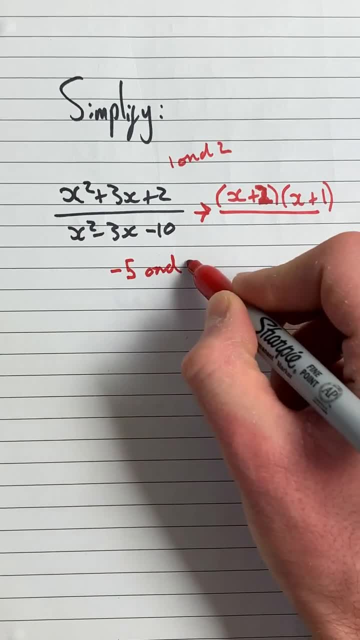 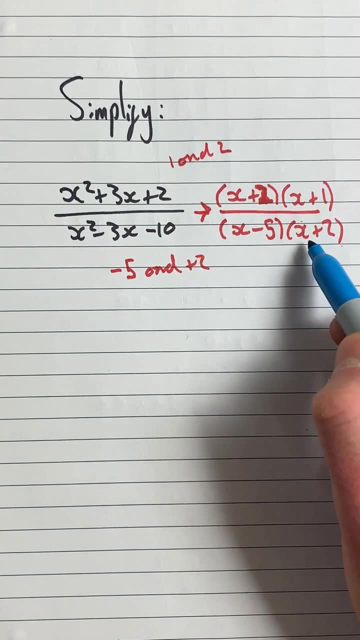 if you think about it for a moment, you'll see that it's minus five and positive two. So the denominator factorises like this: x minus five multiplied by x plus two. After fully factorising you'll notice that we have a factor of x plus two in the numerator and the denominator. so we can. 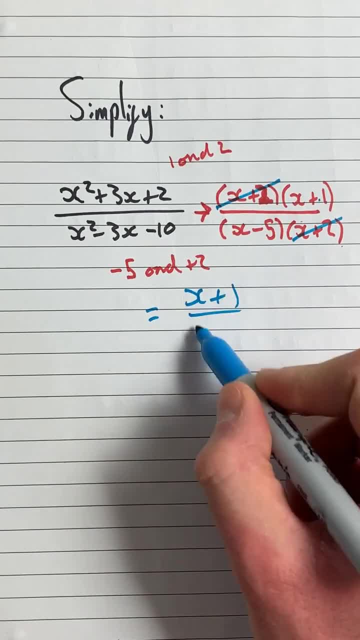 cancel them. This leaves us with x plus one over x minus five and, as a result, this is the simplest form of the algebraic fraction that we started with. 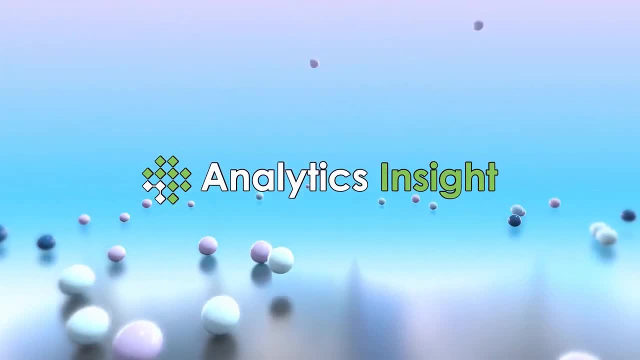 Hello viewers, Wouldn't it be great to know what the future has in store. Predictive analytics is such a progressive technology that leverages big data to predict future outcomes in business. Let us see how the agriculture industry can make the most out of it. 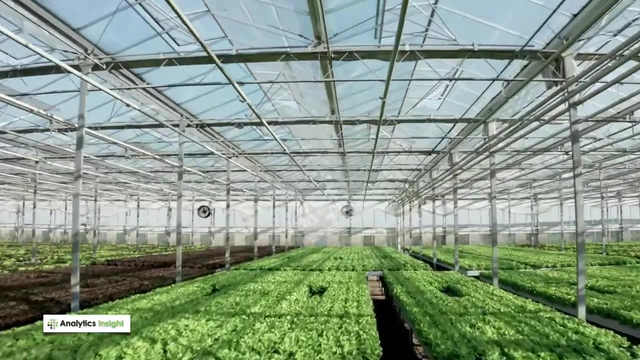 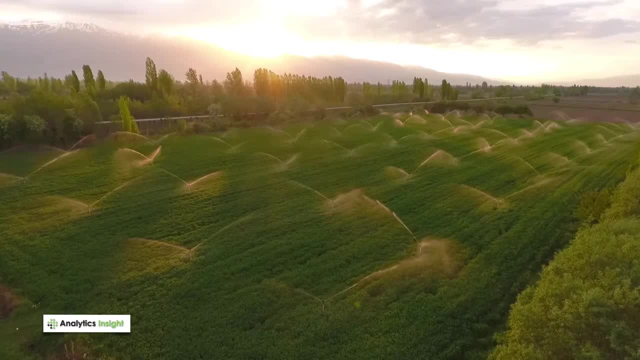 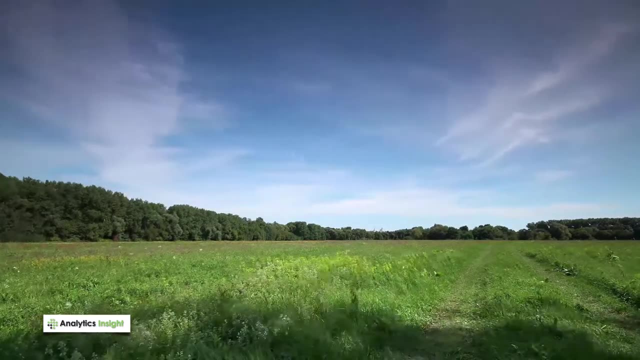 Modern agro-businesses are moving to precision farming to enhance productivity and efficiency. Data provided by in-field sensors help in predicting the amount of resources needed to improve crop quality and yields. The agriculture industry endures the most of climate change. Precision farming using predictive analytics enables to foresee the 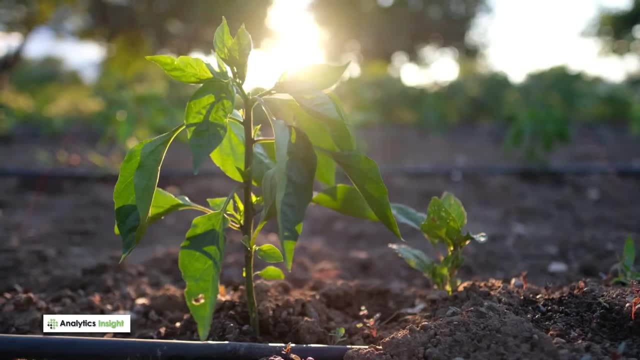 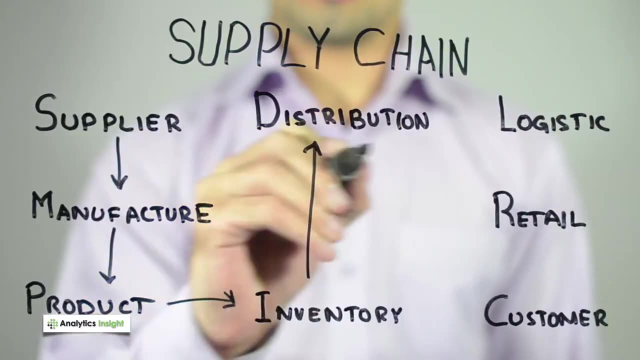 weather conditions for effective resource management and promotes sustainable agriculture. Data-driven agriculture aids in continuous monitoring and enables efficient management of supply chains. Data-driven agriculture helps to improve crop quality and yields. Data-driven agriculture aids in continuous monitoring and enables efficient management of supply chains. 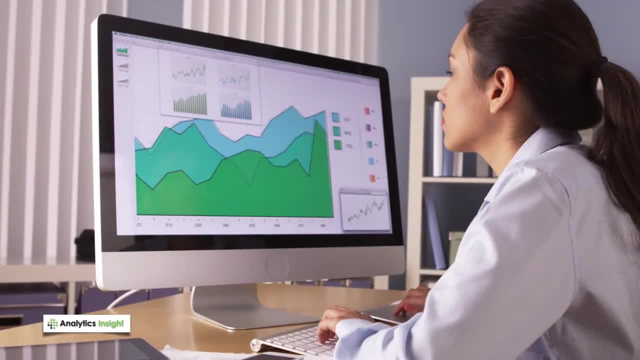 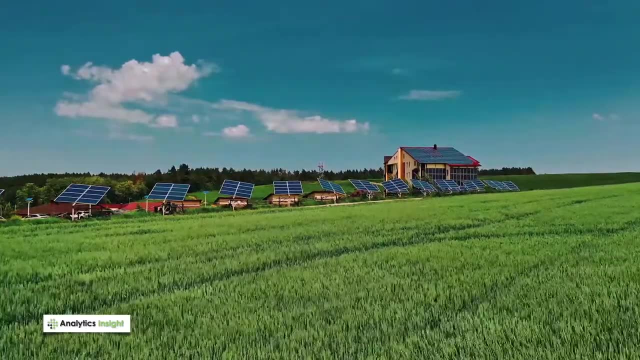 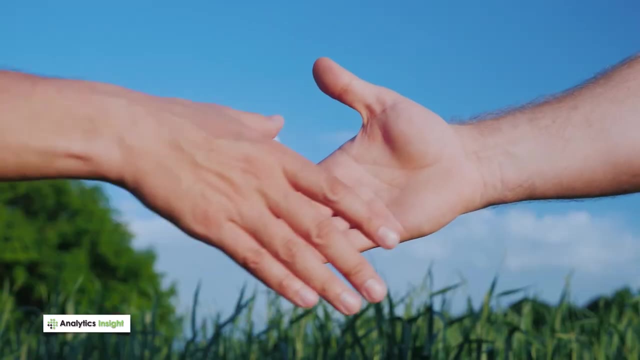 Being able to predict the risks and alternatives ensures better and faster distribution of products. Predictive analytics will enhance the future of agriculture and enable cost-efficient business in the long run. So have you thought of embracing smart agriculture? For more such insights, subscribe to Analytics Insight. 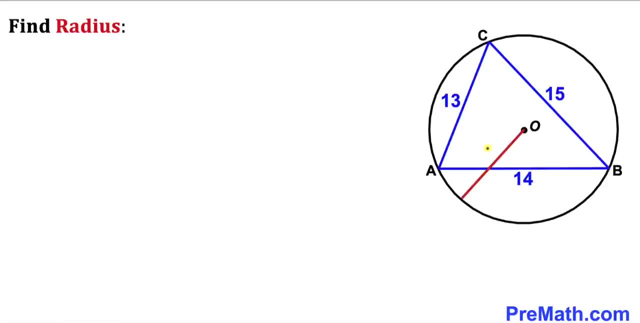 And now our task is to calculate the radius of this circle. Please don't forget to give a thumbs up and subscribe. Please keep in mind that this figure may not be 100% true to the scale. Let's go ahead and get started.